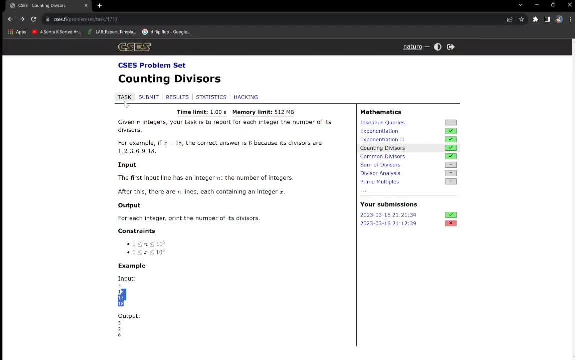 So moving on to the next question, which is counting divisors. So in this task we are given n integers and for each integers we have to calculate how many divisors are there for that particular number. Right, so 16 has 5 divisors, So it is 1,, 2,, 4,, 8 and 16.. These 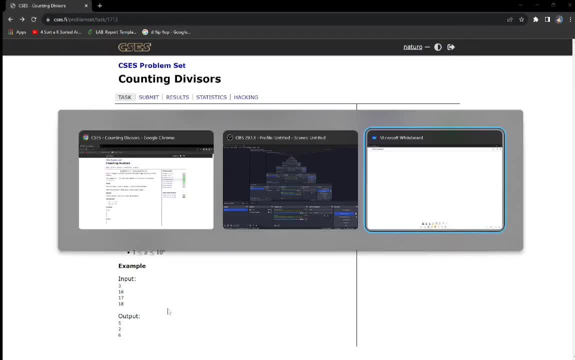 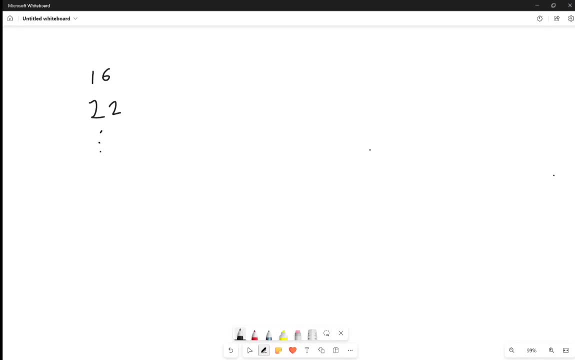 are the 5 divisors. So let us see the intuition behind the problem. So if we give 16,, 22 and likewise so many numbers, right, So what we can do from the very intuitive method, we can apply a for loop and find how many divisors are there for each number. So it 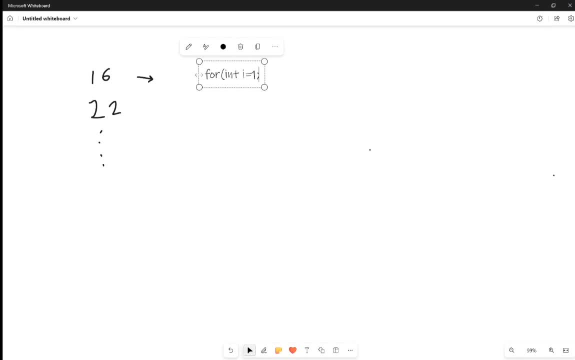 will be like for int, i is equal to 4.. 1,, 2, that number, which is, let us suppose, V of i, right i plus plus, and we will find whether the number is divisible by i or not. So So, 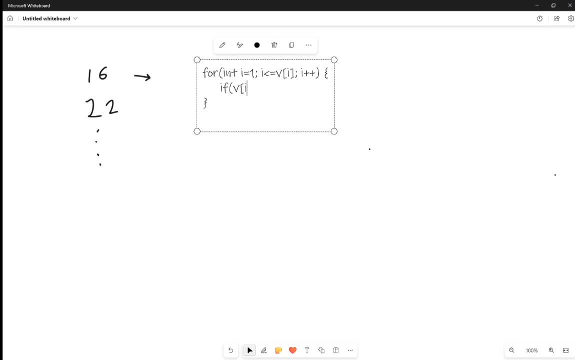 So it will be divisible if V of i modulo i equal to zero, right? So we will increment the counter and at last we will print the count. So this is the very naive approach and the complexity of this approach will be: in each number we are iterating x times because the 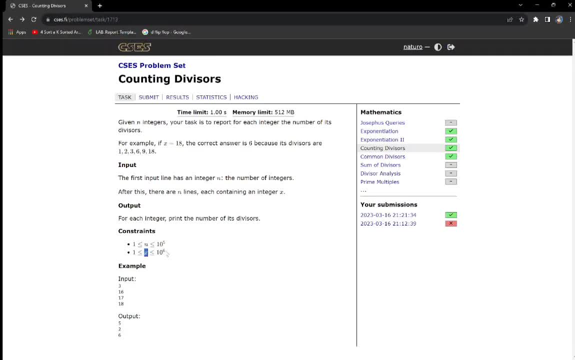 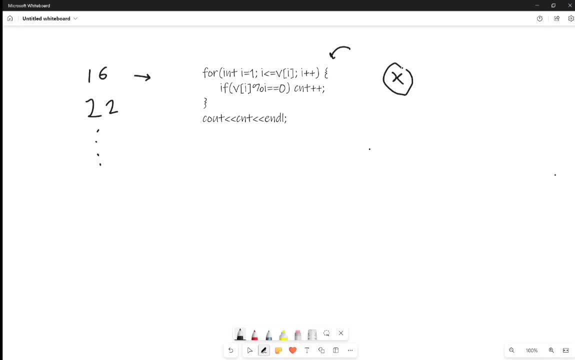 very value of x is 10 to the power 6 and n is 10 to the power 5.. So for each number we are iterating x times and number of numbers are n. So overall time complexity will be big. O of n into x, which is nearly about 10, to the power 5, into 10 to the power 6, which will 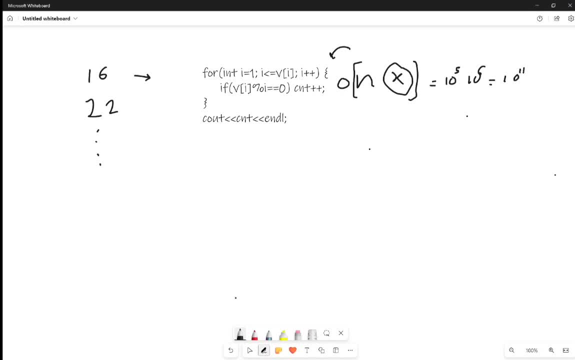 be 10 to the power 11 and it will lead us to a 12.. So that means various product characteristics will be 감AI. So any better optimization we can do. so you must have gone throuuhghlgkhave, which is 9, to the power 6, which will lead. 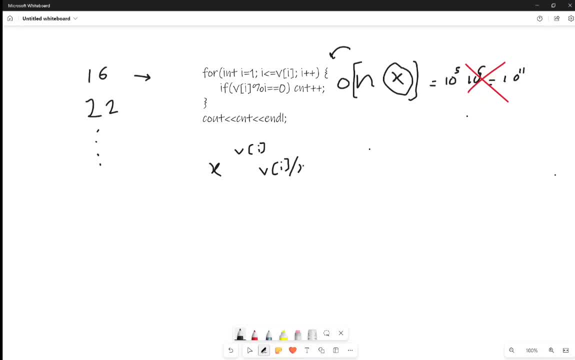 us to a good optimization. Anyway, it works. So any better optimization we can do. so you must have gone through like: if x is divisor of V of i, then V of i by x is also a divisor. let us take an example for understanding this. let us suppose V of i is 6 and 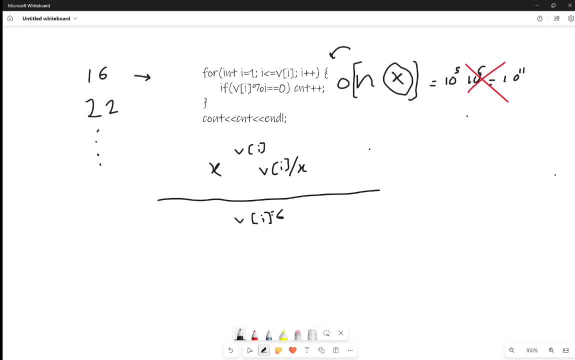 So left axis to RIGHT axis, this is the�so that means this can be our 9 degree earlier. then we canrialised values are 6.. Right opposite is 6.. So any better optimization we can do, so you must have gone through like: if x is divisor of v of i, then V of i is also a divisor we can take. 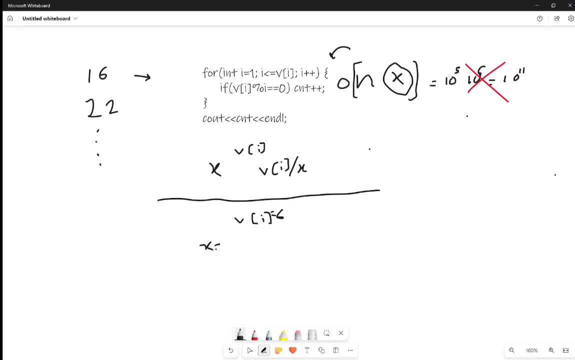 an example for understanding this: let us suppose V of i is 6 and we know that x is equal to 2 is divisor. then it is always satisfied that x by 2 or v of i by x, which is 6 by 2, is also a divisible or divisor of this number. and let us suppose x is something. 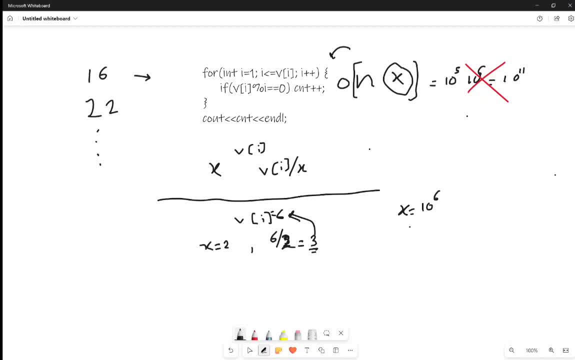 like a big number. so instead of iterating all the numbers, you can just iterate to square root of that number. so square root of 6 will be 10 to the power 3, because let us say the numbers are 1, 2, 3, up to 10 to the power 3 and then 10 to the power 6. 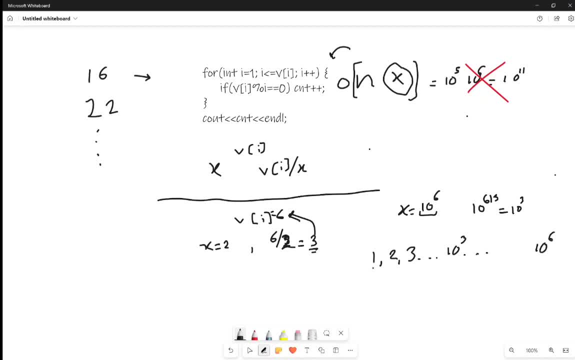 so when we will see that 1 is divisible divisor of 10 to the power 6, then x by this is i, we are it rating from i to 10 to the power 3, then x by i, which is 10 to the power 6 is also divisor. 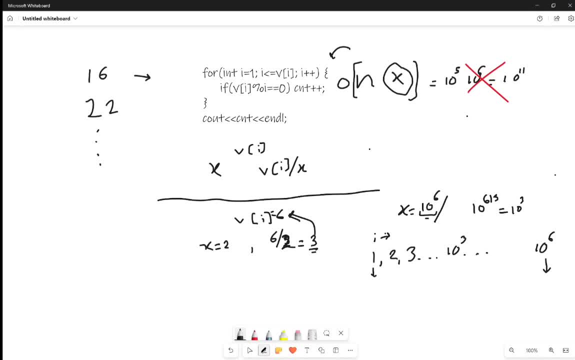 now when we increment our i to 2 and see that i is also a divisive divisor of x, then x by i, which is 10 to the power, 6 by 2, is also divisor of i divisor of x. so 10 to the power 6 will come. 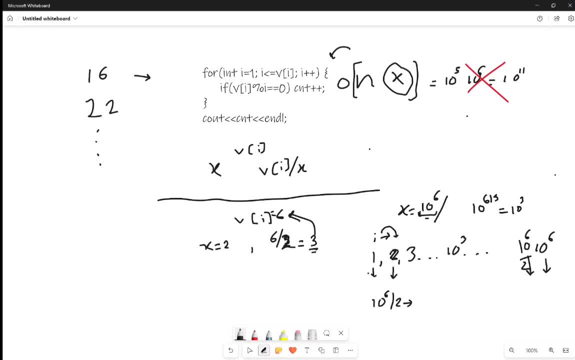 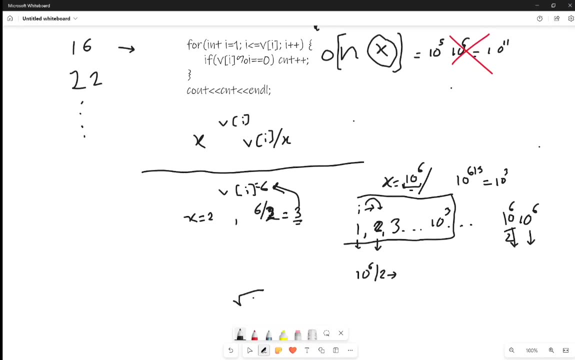 here somewhat here. so we don't have to iterate to all the numbers, we just have to iterate till square root of that number, right? so for each number we have to compute square root of x, and there are n numbers, so complexity will be square root of x into n, which is approximately. 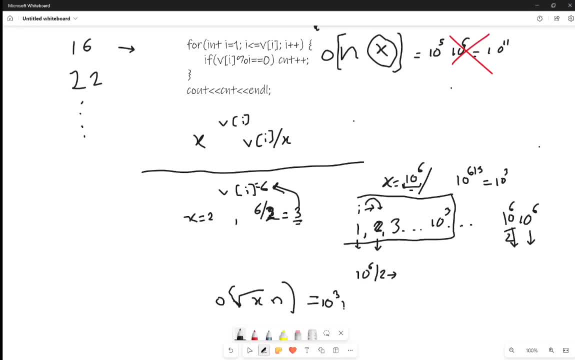 square root of x will be 3 into 10 power 5, so which we? which is again a very great number, because the complexity should be less than or equal to 10 power 7. so it will also not gonna pass our test cases. i have tried this one because 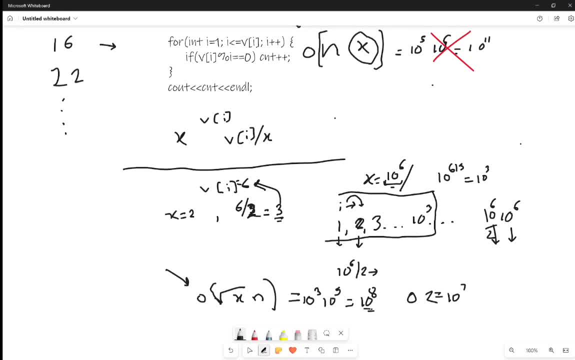 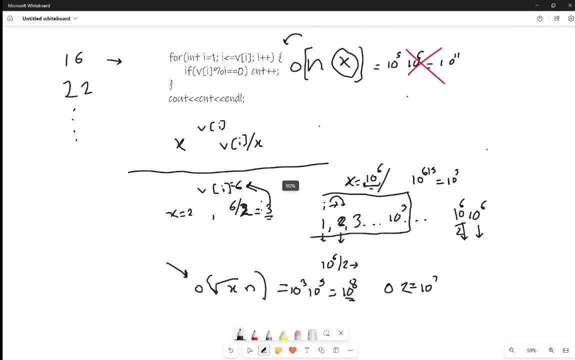 i think that because sometimes 10 power 8 passes in some systems, but here they don't allow, so we have to again optimize it to 10 power 7 or less. Now lets think how it works. Let us see some bit of optimization. So what if we 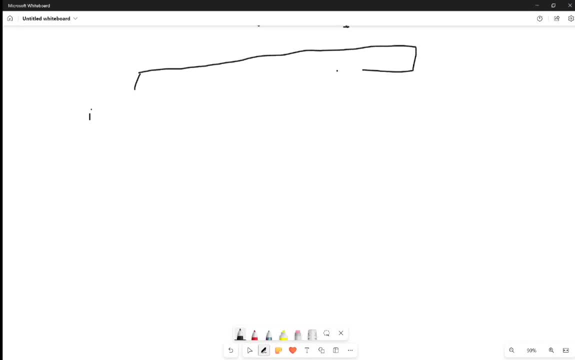 提 lay for each. what if we say of the answers of each number? because the horizon is still ten to the power six, so what if we store the value before answering? This will also not change Because we already page our graphs. three過, So what if we store the value, villa, before answering? 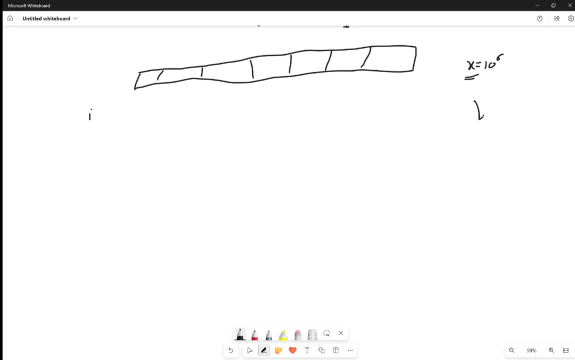 So who has to go with that? so what if we figure out that and just give the value in of one? so let us suppose this is the number one: two, three, four, five, six, seven. we are given n equal to seven and X can be anything. so 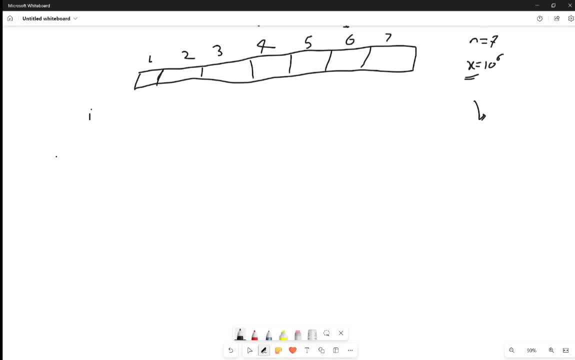 we know that to is divisible DVD with divisor of two. so two is divisor of two, four, six, eight, then and so on. right, so we can increment the divisor of all this numbers. so we will increment divisible of divisor of two. it can increment divisor of four, we can increment divisor of six and so on. so this array will. 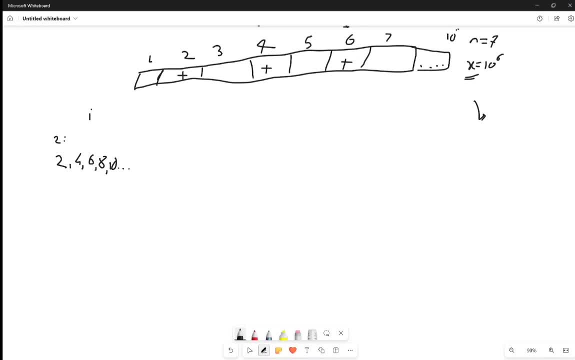 contain already the numbers till 10, to the power 6, because we want to calculate for all the numbers now. we will go for 3, so we will increment. so 3 will be divisor of 3, 6, 9, 12 and so on, so we will increment the. 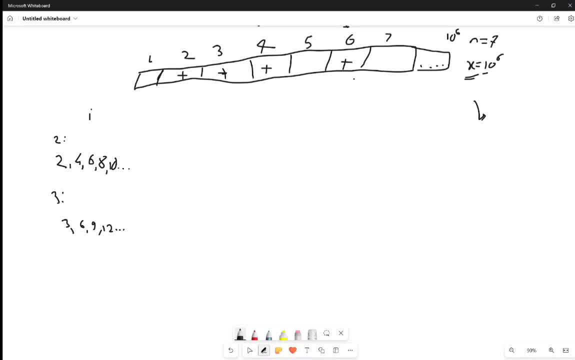 count number of divisor of 3, number of divisor of 6 and so on. likewise, if you go and calculate and store the divisor of all numbers and in next iteration we can just output the number of divisors in O of n. but what's the complexity of this algorithm? because 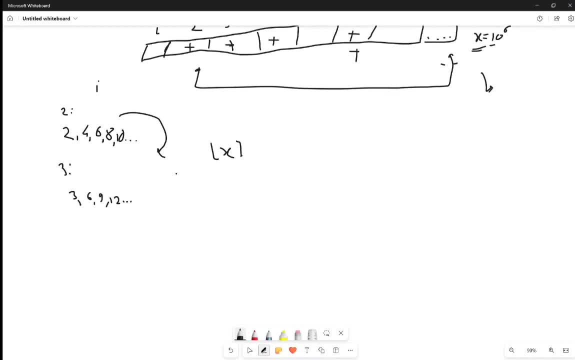 for 2, the number of iterations are x by 2. the number of iterations for 3 are x by 3. similarly, the number of iterations will be x by x. it will start from x by 1 and it will go to x by x, and if you calculate this it will come out to be log of x. so the 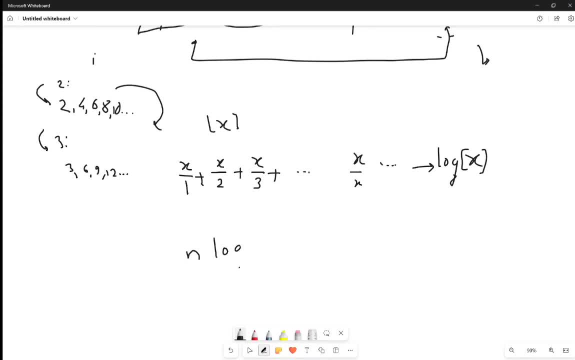 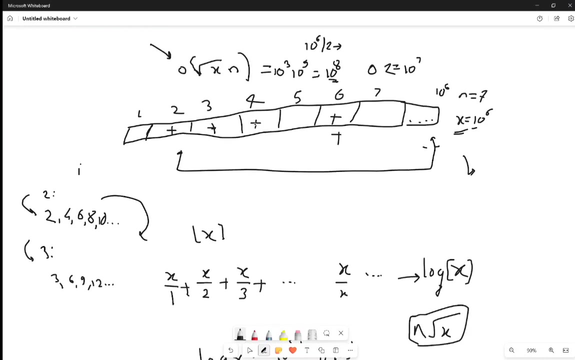 overall time complexity will be n: log of x, which will be around 10, to the power 5, into log of 10 to the power 6, which is very much optimized version of n, into root x. so you have to follow this method. for each number you have to increment the counter from. 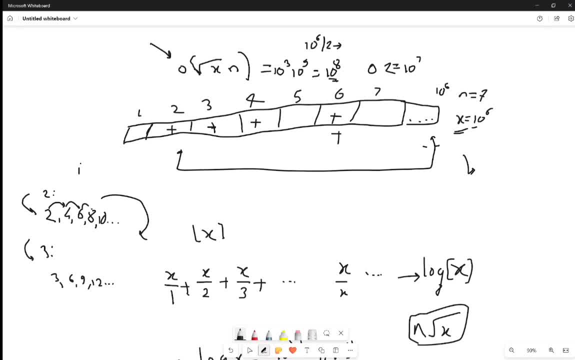 x to the power, from 2, then to 4, then to 6, then to 8, and then for 3, you have to increment the counter by 3. for 4, you have to increment the counter by 4, so number of numbers for 4 will be x. 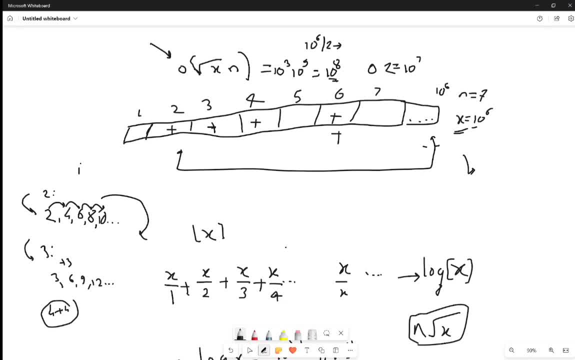 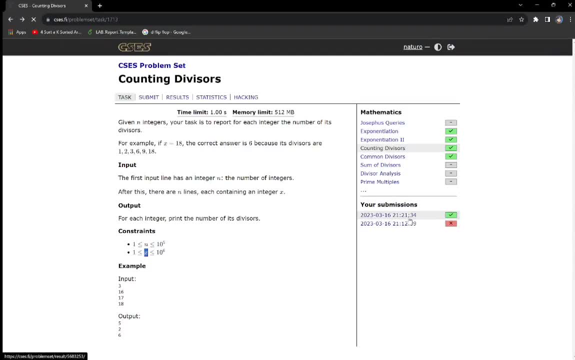 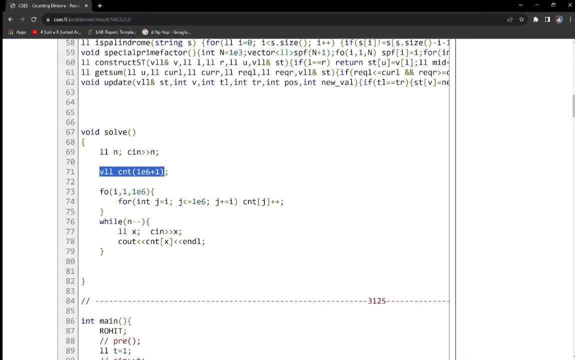 by 4. likewise, you have to calculate, so i will show you the algorithm. so i have initialized a counter variable count vector which will store the number of divisors it has, and i have apply a for loop from 1 to 10 to the power 6 and increment. 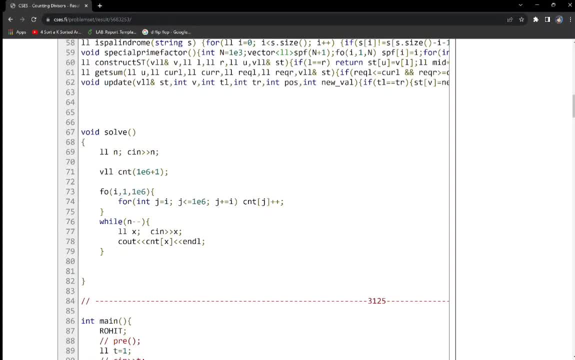 the inner loop by i and increment the number of divisors in the count vector, and for each number, x, i am outputting the number of divisors the x has. so this was the video for today. i hope you liked it and i will see you in the next video. 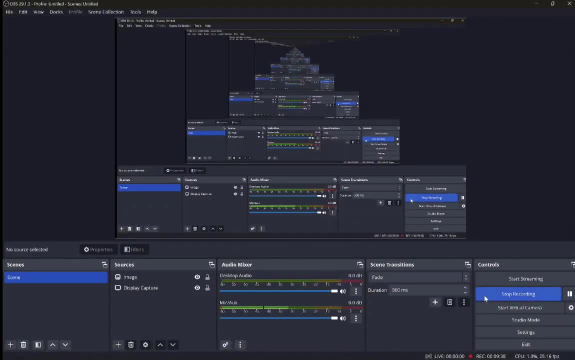 bye, bye. this is the solution of this problem. i hope you like it. thank you very much.